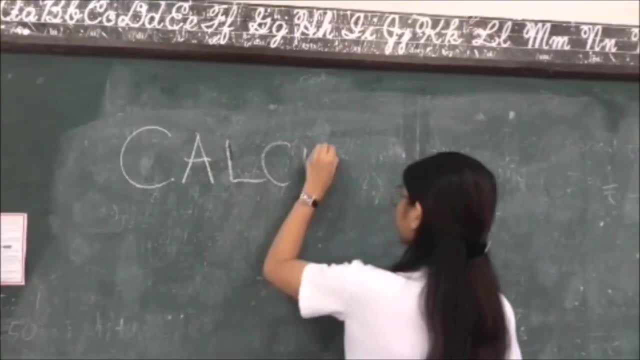 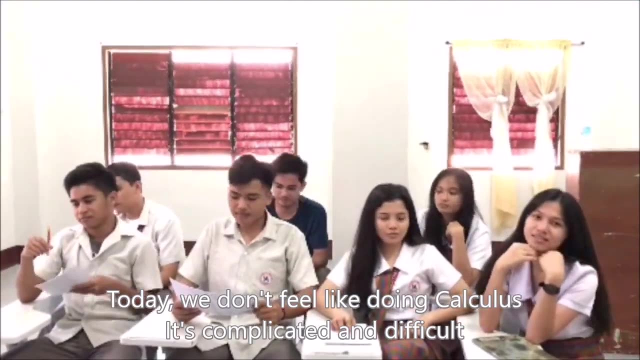 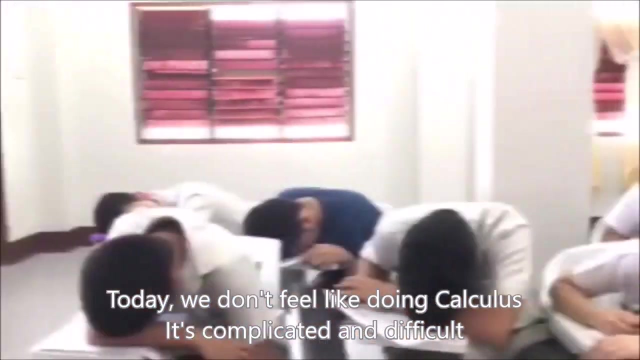 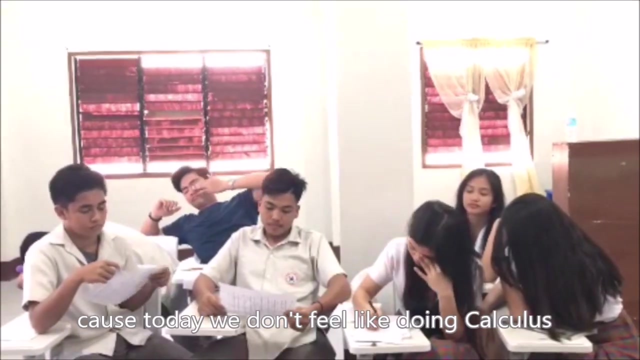 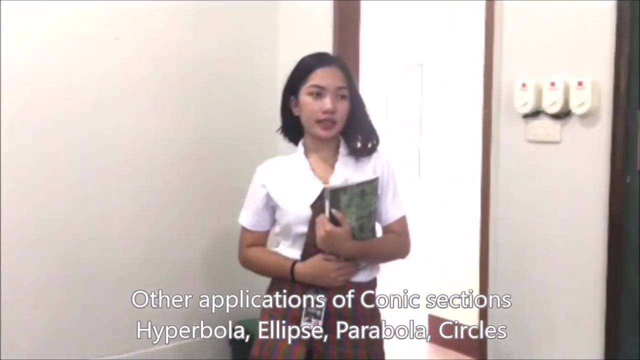 Today we don't feel like doing calculus. It's complicated and difficult. Derivatives in its connect sections showing graphic solutions. But today we don't feel like doing calculus. Are there applications of connect sections: Hyperbola, ellipse, parabola, circles, Could. 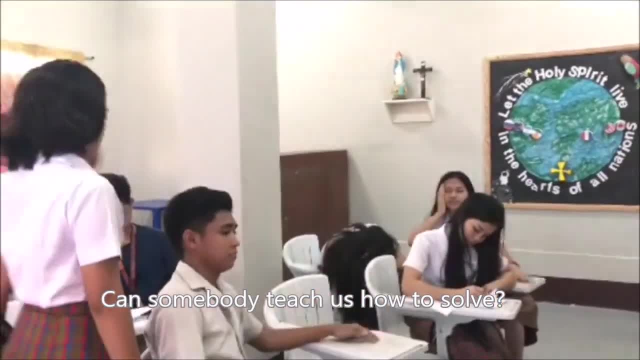 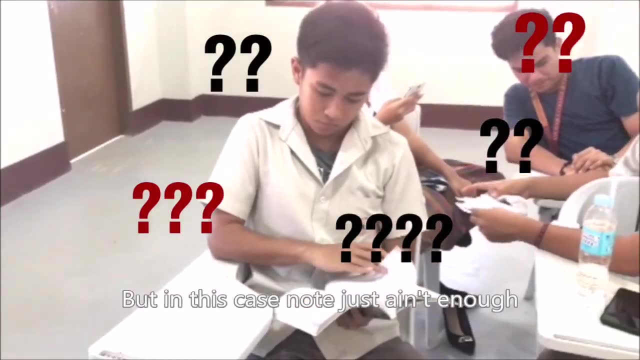 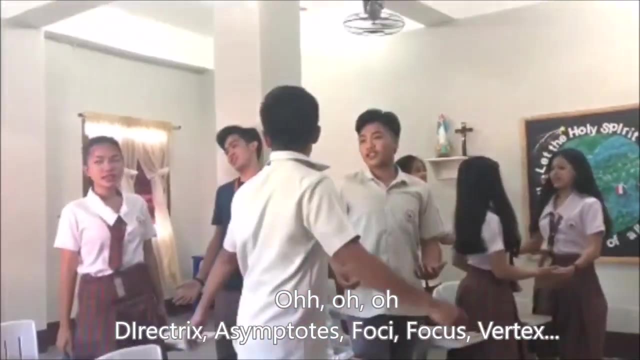 somebody teach us how to solve. We'll be sitting on the couch just chilling with our studies, flipping through our notes, hoping that it would help us, But in this case notes just ain't enough. Oh, direct checks of symptoms for sight focus vertex. Today we don't feel like doing. 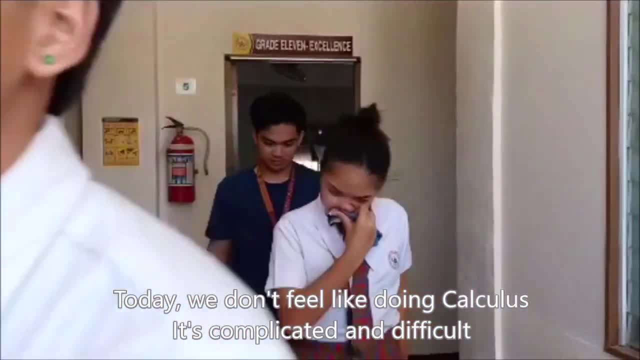 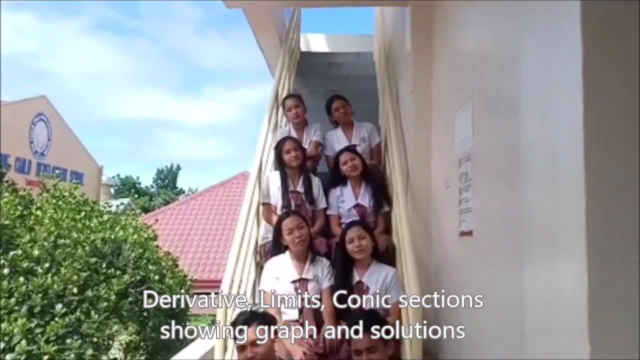 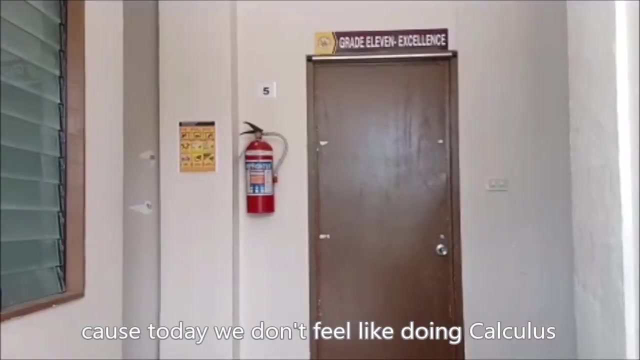 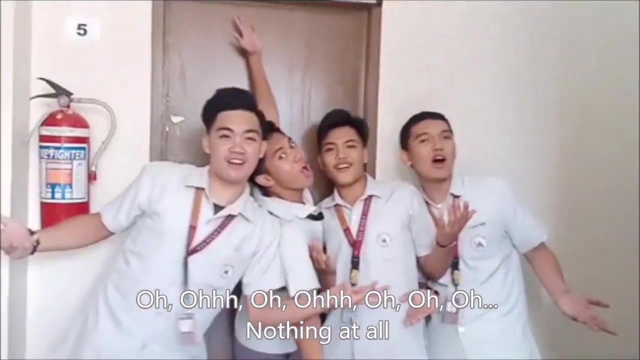 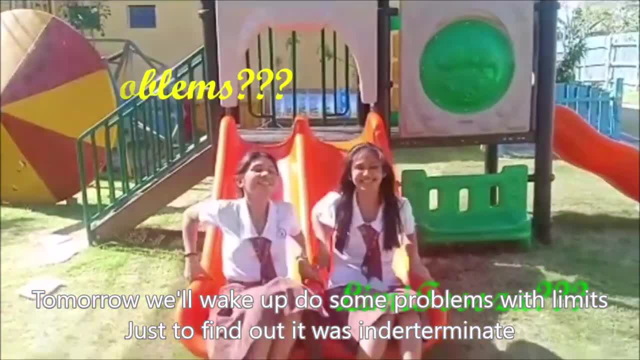 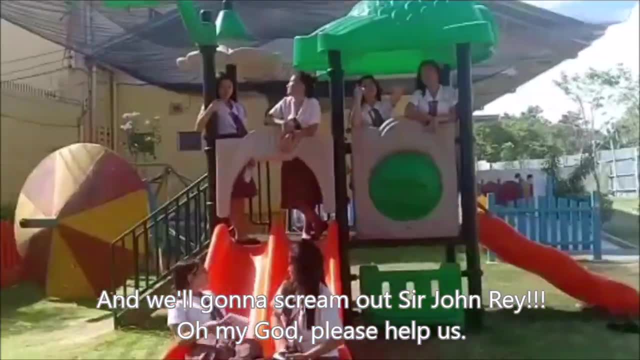 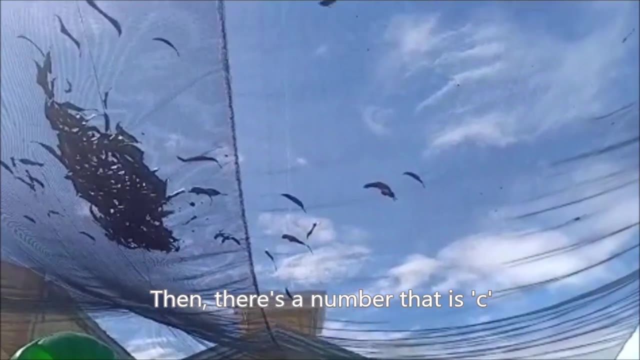 Tomorrow we'll wake up to some problems with limits. Just a flat note: that was indeterminate. We'll wanna scream out: surgeon way, Oh my god, please stop us. We might use a run with some ambiguity: Define continuous differentiability, But there is. 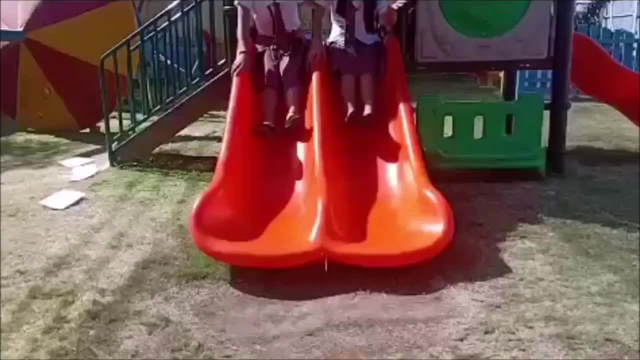 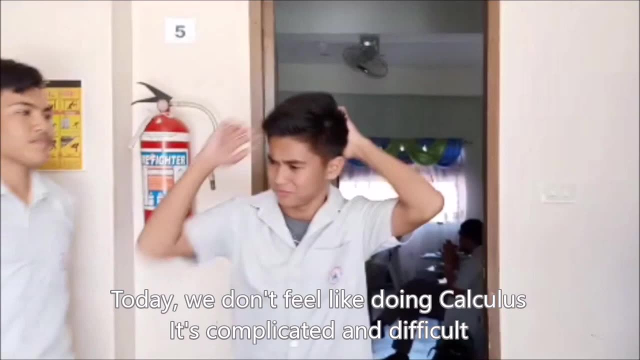 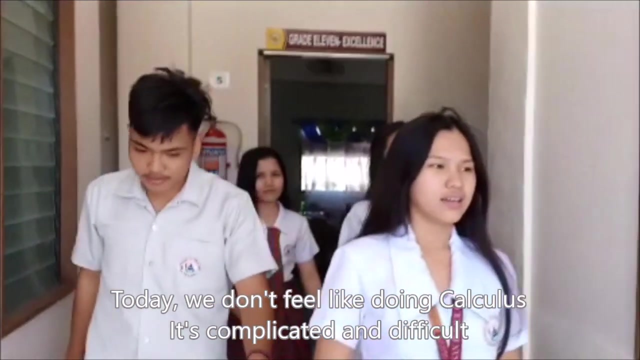 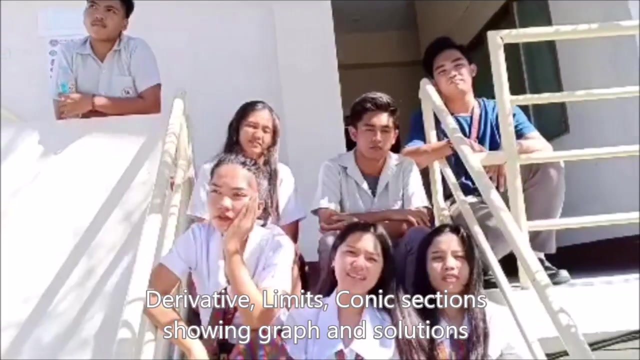 a number that I see, Oh, F of 65,. limit exists, continuity: Today we don't feel like doing calculus. It's complicated and difficult, Derivatives in its connect sections showing graphic solutions. But today we don't feel like doing calculus. 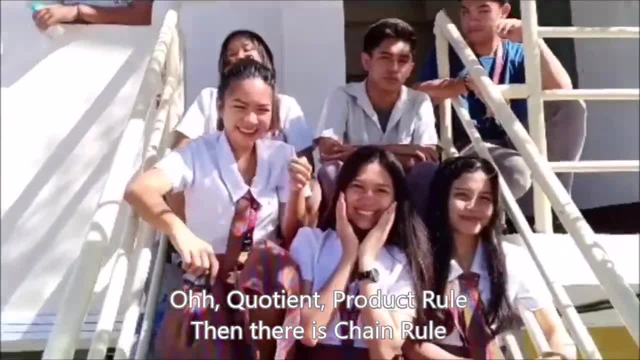 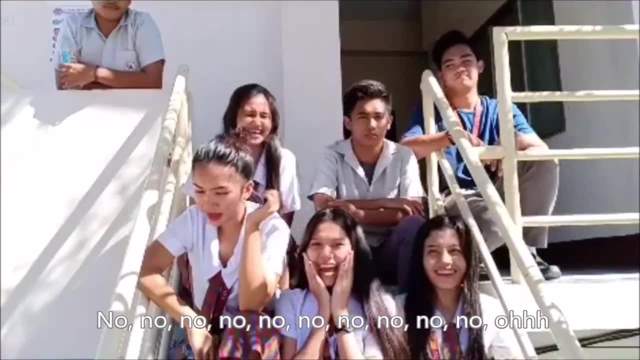